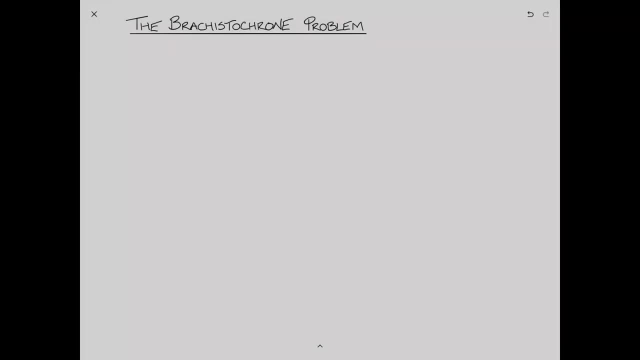 The Brachistochrone problem is a hugely important problem in the world of variational calculus and therefore in the world of classical mechanics too. This problem was first posed as a challenge by Johann Bernoulli, and it was more than just a problem that he posed, I mean, there was far-reaching 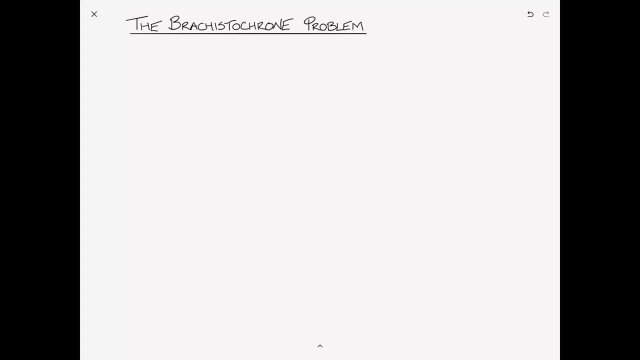 politics behind this. The meaning of the word Brachistochrone comes from the ancient Greek meaning shortest time, and it describes a problem in which we're given two points. we'll call the first a at a location x1- y1, and b at a location x2- y2, and the idea is that, under the influence 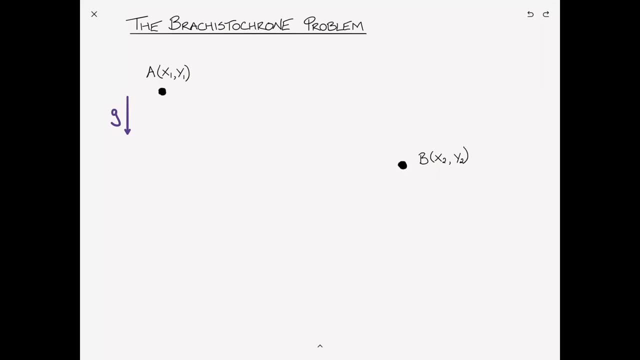 of gravity, what is the shape of the curve between the two points that would cause, say, a marble, rolling down that slope to get from a to b in the shortest time? and, following one's intuition, one might use as the starting point a straight line, because, after all, a straight line is the 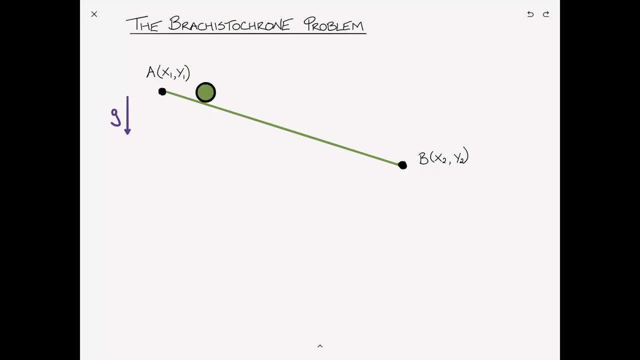 shortest time. So the idea is, if we have a marble here, say, that's rolling down this frictionless path under gravity, can we perhaps find a better, a more optimal path that will cause this marble to get from a to b quicker? So let's have a look at the actual statement of the problem as it was originally. 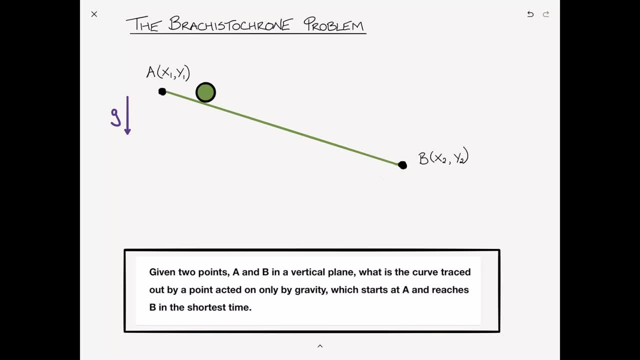 stated: Given two points, a and b, in a vertical plane, what is the curve traced out by a point, acted on only by gravity, which starts at a and reaches b at the shortest time? and the idea is that we might have a marble that's rolling down this frictionless path under gravity, and that's. 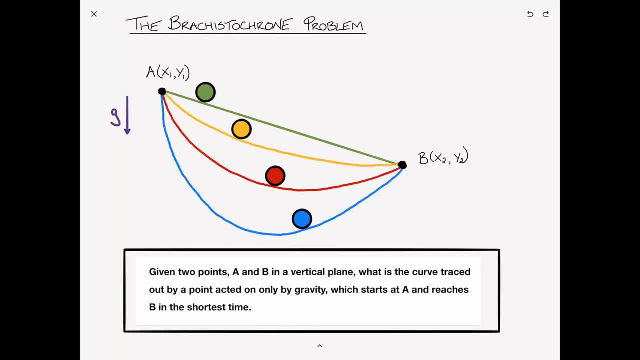 why it's called a straight line. So if we have a marble that's rolling down this frictionless path under gravity, we might consider a whole assortment of different paths. Can we determine which one of these paths would take the shortest time? Back in the 1600s, the late 1600s, the mathematicians of 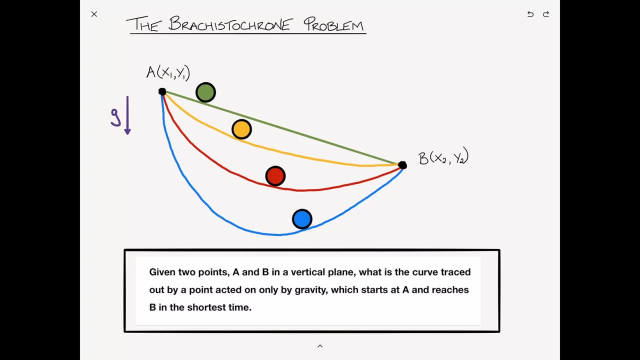 Europe believed that they were the smartest in the world, and it was not uncommon for mathematicians to pose problems in publications as a way of advancing research. In the case of the brachistochrone problem, the problem was posed by Johann Bernoulli in 1696, with an announcement that went as follows: 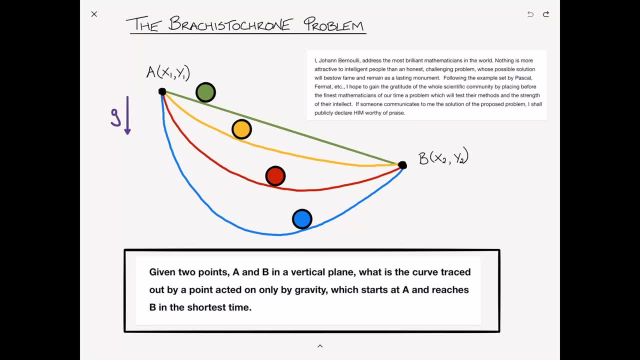 I, Johann Bernoulli, address the most brilliant mathematicians in the world. Nothing is more attractive to intelligent people than an honest, challenging problem whose possible solution will bestow fame and remain as a lasting monument, Following the example set by Pascal, Fermat, etc. 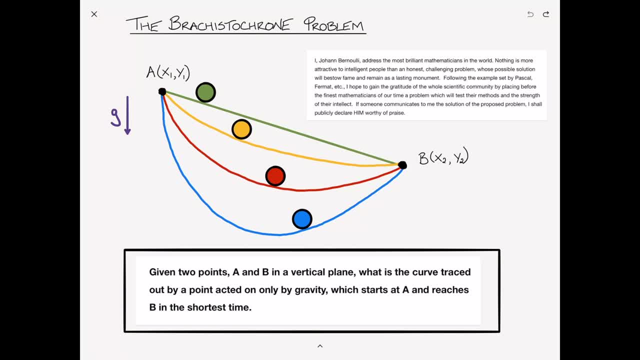 I hope to gain the gratitude of the whole scientific community by placing before the finest mathematicians of our time a problem which will test their methods and the strength of their intellect. If someone communicates to me the solution to the problem, I will be able to answer. 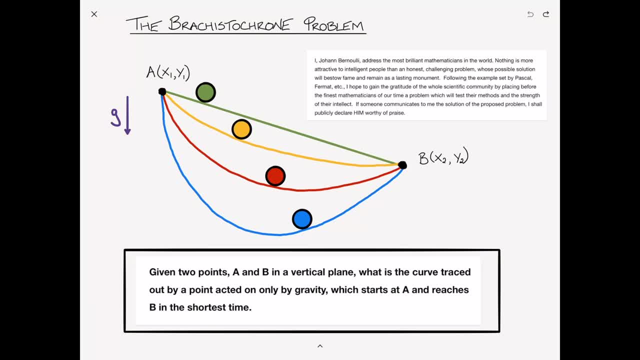 the question of the proposed problem, I shall publicly declare him worthy of praise. I guess women need not apply back in the 1690s. Before I start on the solution to the problem, a little bit of the history first. Let's have a look at a timeline and, like any good timeline, we'll start. 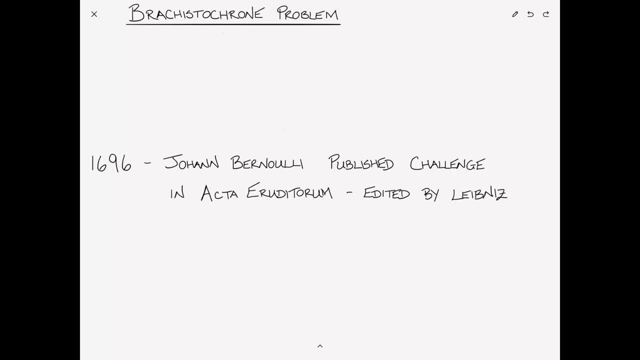 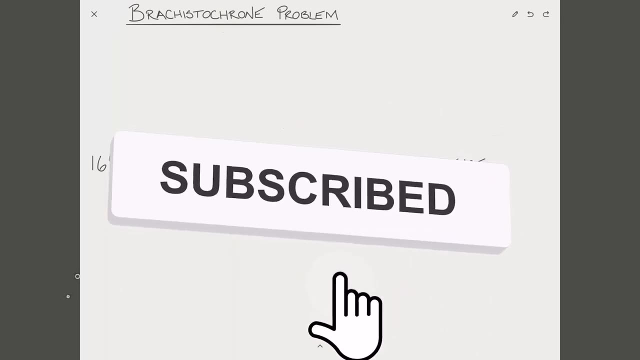 in the middle, so we can go forwards and backwards from there. In 1696, Johann Bernoulli published this challenge in a journal called Acta Eruditorum, which so happened to be edited by Leibniz, and he posed this problem as a challenge. 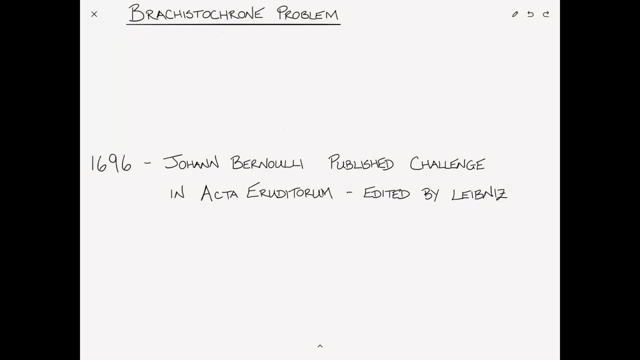 To the mathematicians, but really what they're trying to do was to bait Newton. There was huge animosity between Leibniz and Newton because of what had gone on with the invention and the credit taken for calculus. And Newton at this point was an elder statesman, He was in his 50s. He had 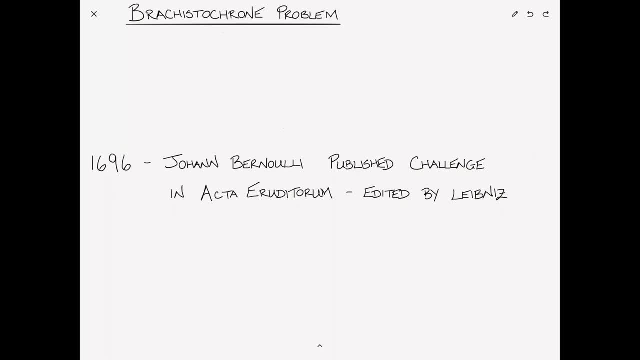 retired from being a professor and was now warden of the mint, which is something like today's equivalent of secretary of the treasury, A position that he would hold on to for the next 30 years, until his death. So despite the fact that Newton would go on to live to a ripe old age, 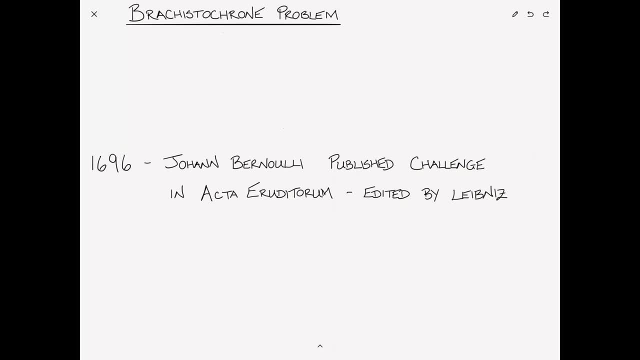 into his 80s, and despite the fact that he was the greatest scientist that had ever lived on this planet, science at this point had become a side gig for him. Johann Bernoulli was a man of about 30, and he and Leibniz were keen to egg on Newton, especially since Bernoulli had already found 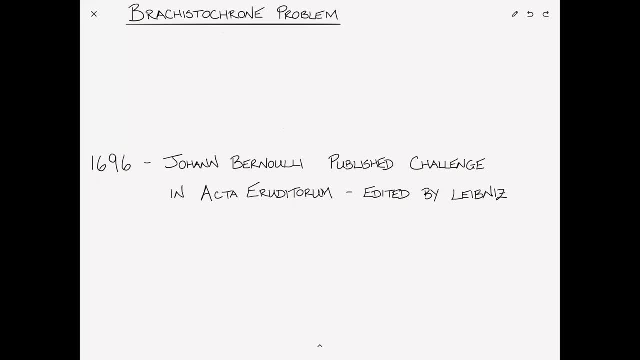 the solution to this problem. In a fitting bit of irony, his solution was actually wrong, or perhaps rather than wrong, it contained an error and his brother's Jacob was correct. but more on that in a bit. Bernoulli's mathematical challenges in journal publications was nothing new, In fact about 50. 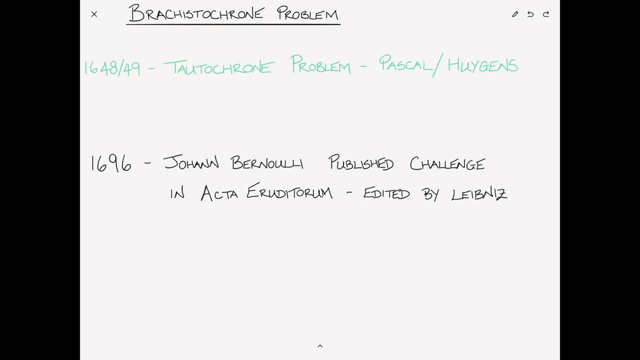 years before that, in 1648, the Tautochrone problem, which is a related problem to the Brachistochrone problem. We'll talk more about that later, but this was a problem that was posed by Pascal in a journal and it was solved by Christian Huygens. Now, actually, Bernoulli was. 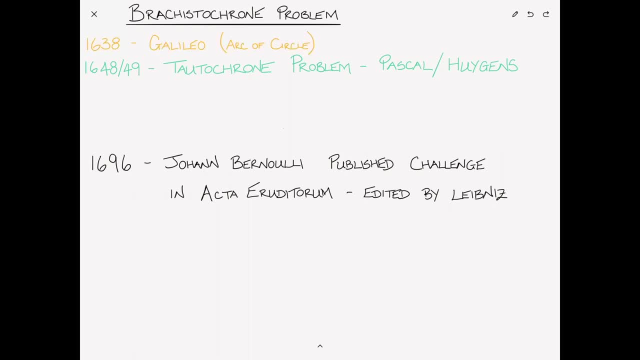 not the first one to weigh in on the Brachistochrone problem. Back in 1638, Galileo had actually had something to say about it, and he got it wrong. He thought that the best way to solve it was to use a curve. The best curve was the arc of a circle, but he was able to successfully demonstrate 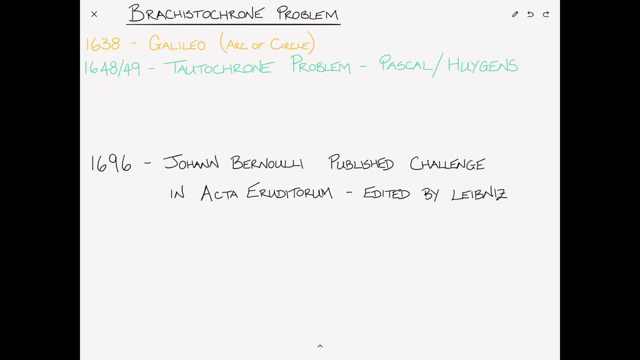 that a curved path was more optimal than a straight path. This challenge was posed in about the middle of 1696, and six months later they had received six solutions. Five of those solutions were from household names. I guess, if your household is run by mathematicians Solutions. 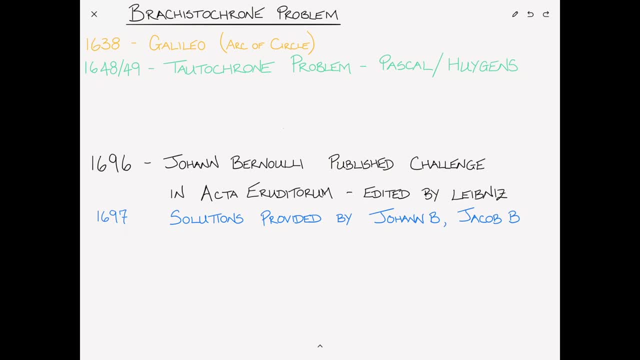 were provided by Johann Bernoulli, by his brother Jacob Bernoulli, by Lopi Tal, who happened to be a student, a PhD student, of Johann Bernoulli's, And then, of course, they were successful in egging on Newton. So just to give a little bit of 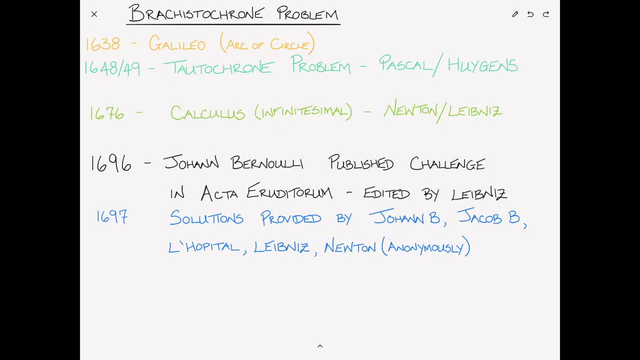 background in terms of the science and theory that was available at the time. Newton, in 1676, had published calculus- he and Leibniz independently- And about 11 years later, in 1687, was when Newton published his Principia Mathematica, which included his laws of motion and universal gravitation. 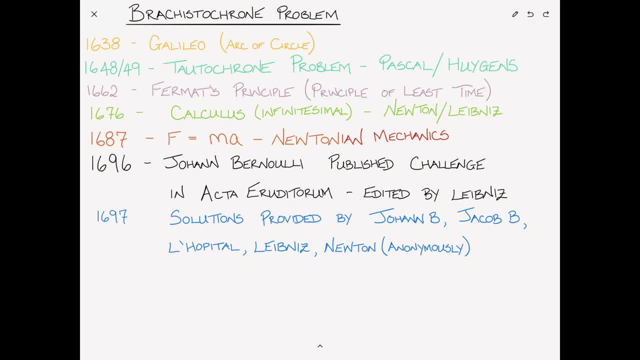 But the Bernoulli solution actually relied on Fermat's principle, which was published back in 1662.. It's also known as the principle of least time And interestingly- and I suggest all of you read up on this because it's fascinating- in traveling from point A to point B, light will always follow. 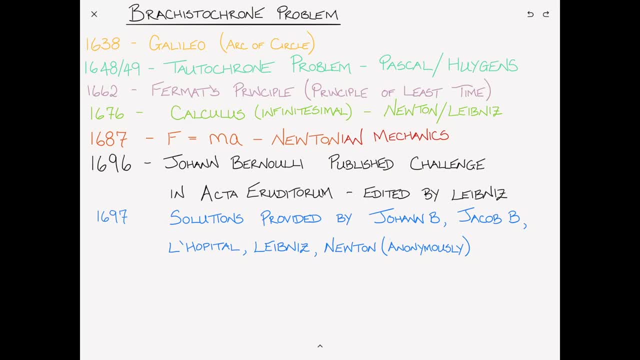 a path that gets it from point A to point B in the least possible time, And hence the first flavor of a path minimization type problem. And using this principle, Johann Bernoulli was able to come up with a solution, A very elegant solution, mind you, despite containing an error which was later fixed. 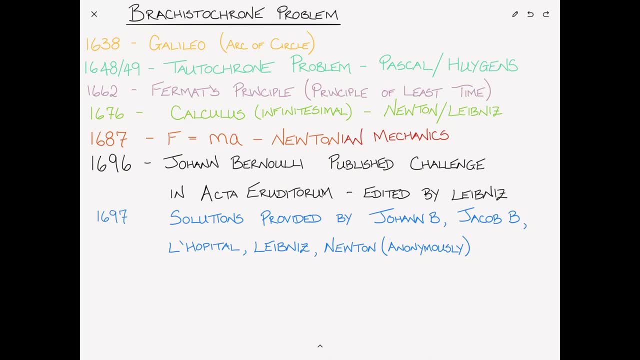 So Jacob Bernoulli was able to come up with a solution, which was later fixed. So, Jacob Bernoulli, Jacob Bernoulli produces a correct solution, also using Fermat's principle, And Johann Bernoulli tries to pass off Jacob's solution as his own. Well, you can imagine the fireworks that ensued. 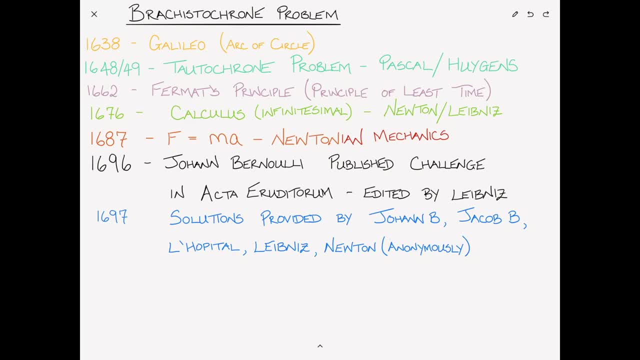 The Bernoulli brothers were competitive, to say the least, and were trying to outdo one another constantly, even though there was 12 years separating them. In an attempt to outdo his brother, Jacob, Bernoulli ended up creating a harder version of the Brachistochrone problem. 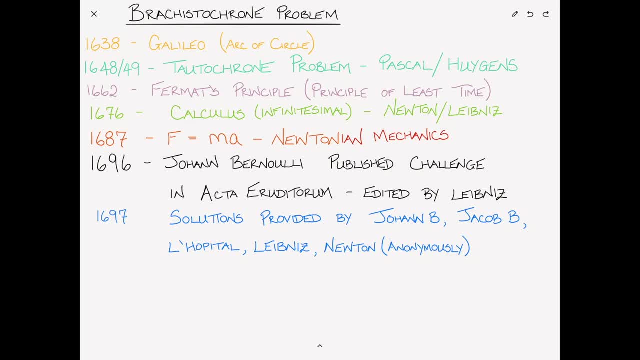 And in solving it, new methods were developed and designed by Euler, which later became the calculus of variations. Unfortunately, Jacob Bernoulli would die at age 50, only eight years later, and it would never get to see much of this calculus. 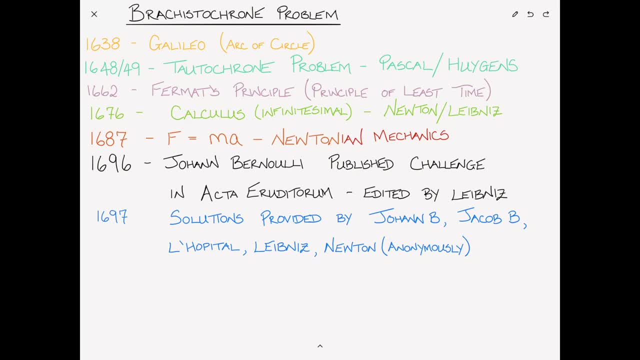 of variations materialize. So the story goes that it took Johann Bernoulli two weeks to come up with his solution And Newton, after coming home from the mint one day at 4 pm, decided to sit down and solve this, And by 4 am the next morning he had come up with a solution And Newton had 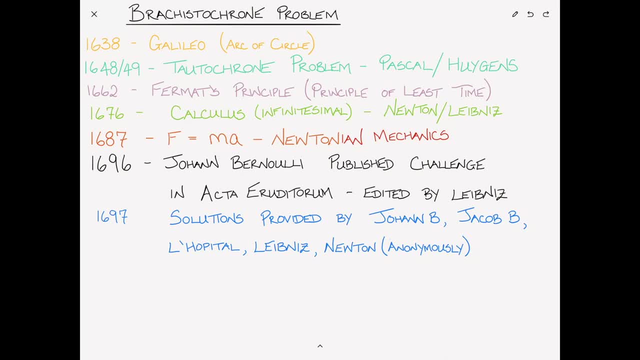 already solved Newton's minimal resistance problem, which is considered to be the most effective solution. So it took Newton all of about 12 hours, And although Newton published his solution anonymously, it is said that upon seeing the solution, Johann Bernoulli exclaimed: 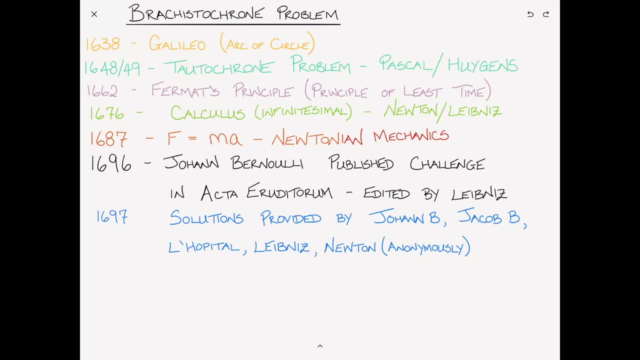 I recognized the lion by his claw mark. Okay, so this gave rise to the Brachistochrone problem, And then, about 10 years later, Leonard Euler is born. For those of you who are not exactly aware of this, Leonard Euler is perhaps the best mathematician in history. 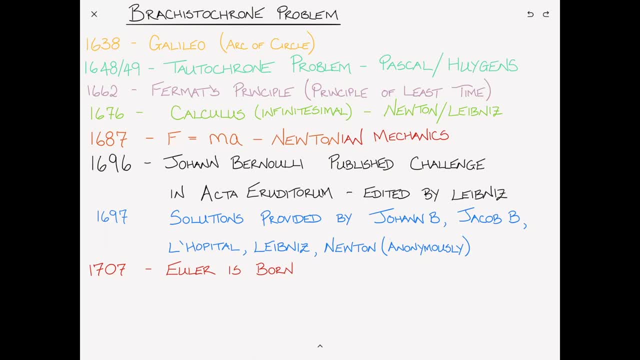 Certainly the most prolific, having published over 900 books. He was said to write about 800 pages a year. So Euler is born in 1707.. Euler is Swiss and is obviously influenced by the Swiss mathematicians. And in 1726, Euler completes his PhD. And who is his advisor? Johann Bernoulli. 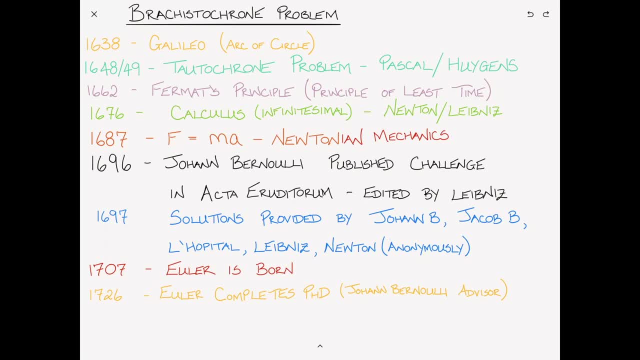 His PhD deals with the propagation of sound. It's actually not at all related to the Brachistochrone problem. But then in 1733, he starts working on the Brachistochrone problem And he's a problem. In 1755, along comes Lagrange, age 19.. He's working on the Tortochrone problem. Yes, 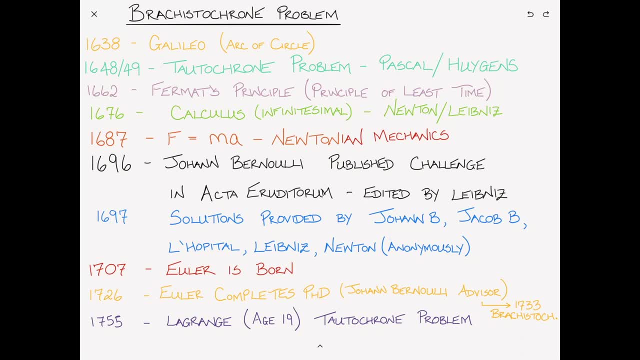 that Tortochrone problem from back in the 1640s. He writes a letter to Euler explaining something he's come up with. His solution is purely an analytical one and is different from the solution Euler is working on. Euler is so impressed by what Lagrange presents him that he stops his work. He 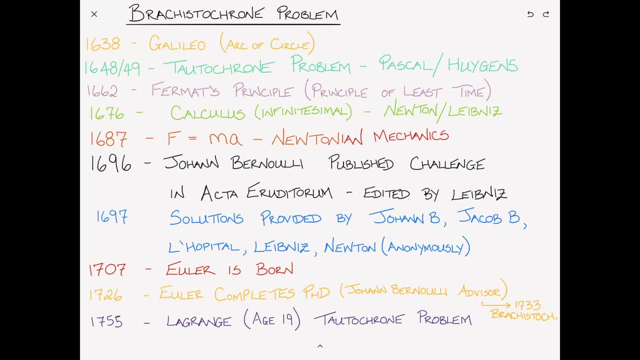 realizes Lagrange has it correct. Let me give him some time to catch up. Lagrange, by the way, while not quite the mathematician Euler was, was the master of mechanics, as you're probably beginning to realize. He just was a real prodigy and had a feel for. 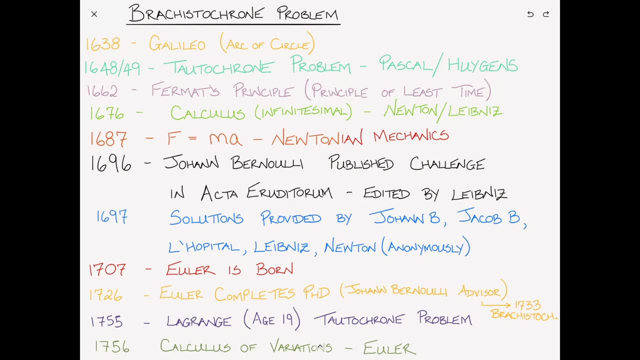 things. And then, finally, in 1656,, Euler publishes the Calculus of Variations, which provides a framework for Fermat's principle, for the Tortochrone problem, for the Brachistochrone problem and a whole bunch of other path minimization problems Newton lived well into. 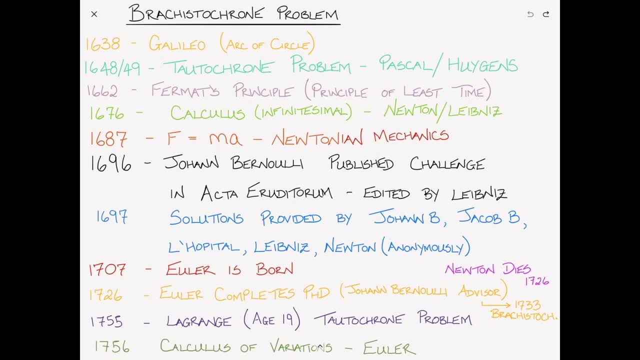 1726, at about the same time that Euler was completing his PhD. So unfortunately, he would never get to see the Calculus of Variations, although one kind of feels like maybe he had it in his head all along. Okay, so Johann Bernoulli solved this in two weeks. Newton solved it in 12. 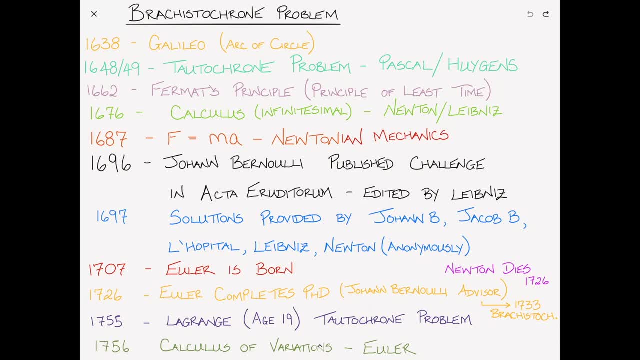 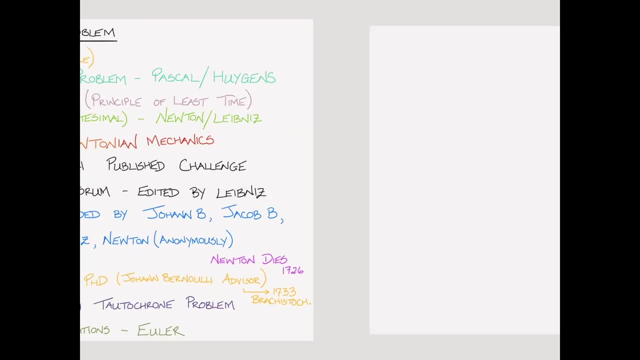 hours. I'm going to solve this for you in the next 10 minutes, But, to be fair, I have something on my side that none of these guys had. I'm going to use the Calculus of Variations. Okay, so let's get on. 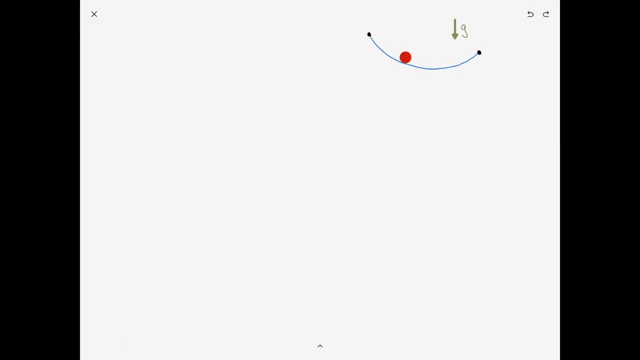 with it The Brachistochrone problem. We've got points A and B and, under the influence of gravity, a marble is going to roll down this frictionless path. From my experience working with this problem, I find that the math comes out the cleanest if we set up our coordinate system. 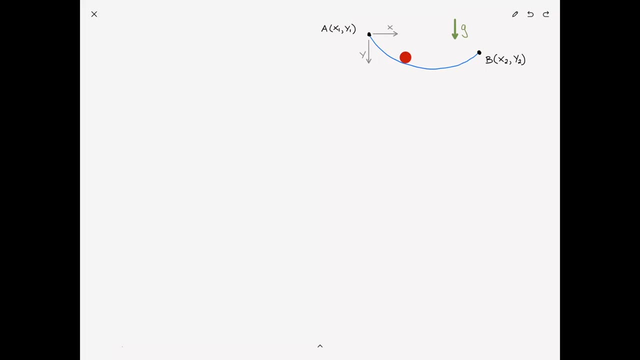 as follows: with the origin at point A and the x-axis in its usual direction, pointing to the right, but the y-axis pointing down, Proceeding within the framework of the Calculus of Variations, what we're trying to do is set up an integral I. 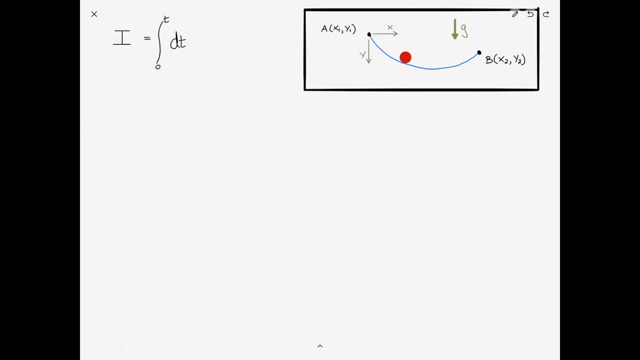 call the time taken. We want to minimize the integral from 0 to t of dt. Now, the time taken can also be written as the integral from point A to point B of ds, the incremental path length divided by the velocity, And we'll call this equation 1.. Now, in order to get an expression for both ds and the 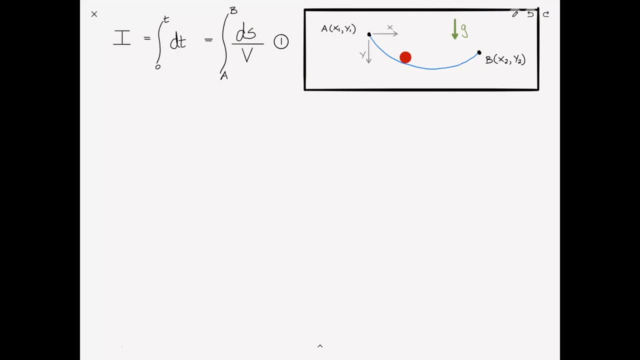 velocity v. we can come up with an expression for the velocity v by using the conservation of energy. The kinetic energy of the marble is one half mv squared, and that is equal to the loss in potential energy. Now, because I've defined the y-axis as 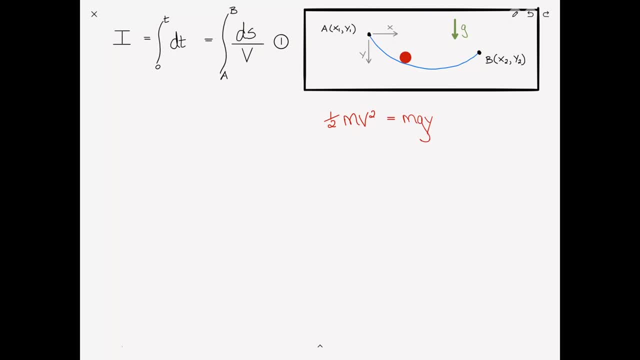 pointing downwards. that's just equal to mgy. The kinetic energy of the marble is equal to its loss in potential energy, And this can be solved for the velocity equal to the square root of 2gy, To come up with an expression for ds. I've shown this in several videos before. there's a link. 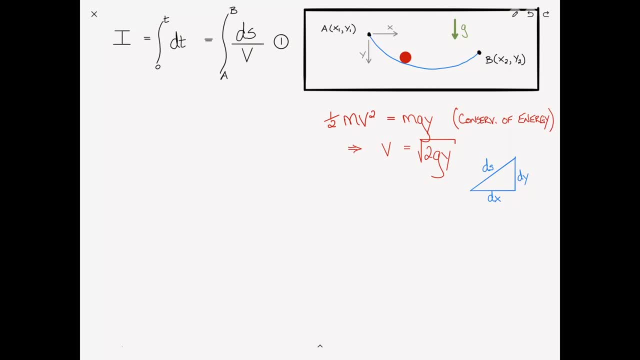 to that. above we look at an incremental path length ds. It has a horizontal component, dx, and a vertical component, dy. Then we, by Pythagoras, we can write that ds squared equals dx squared plus dy squared, and this gives us an expression for ds is equal to the square root of 1 plus y, prime squared dx. Let's give these some. 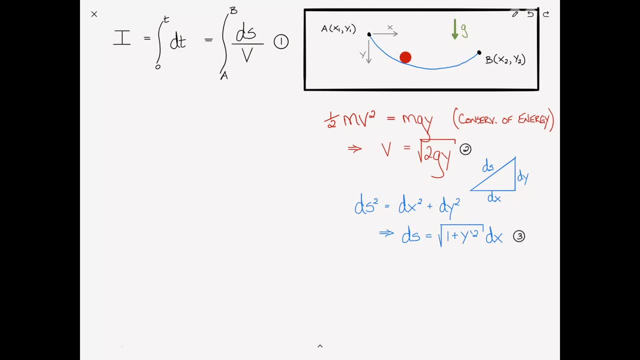 numbers 2 and 3. and now what we want to do is substitute 2 and 3 into equation 1.. So substituting yields the integral from x1 to x2 of root 1 plus y prime squared dx, that's just ds divided by the. 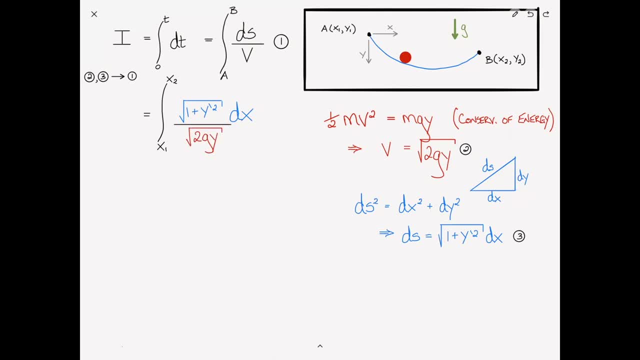 velocity, which is root 2 gy. I can simplify this by taking 1 divided by root 2 g to the outside times, the integral from x1 to x2 of root 1 plus y prime squared divided by y dx. From this we can: 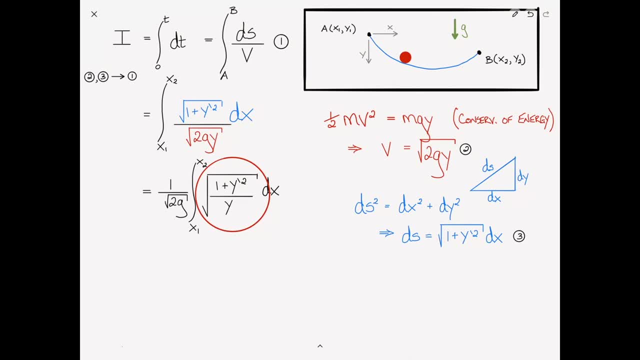 see that the functional in this case is just this pass here. So f is just root 1 plus y, prime squared divided by y. Let's number these 4,, 5, 6, and I've shown in a previous video that a link to that appears above that. in the event that our functional doesn't explicitly depend on x, 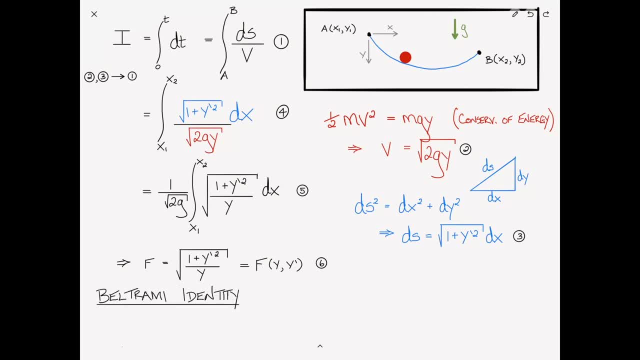 the Euler-Lagrange equation reduces to something known as the Beltrami identity. The Beltrami identity states that f minus y prime times partial f, partial y prime is equal to a constant, and that is equation 7.. So all I need to do now is substitute equation 6 into equation 7. 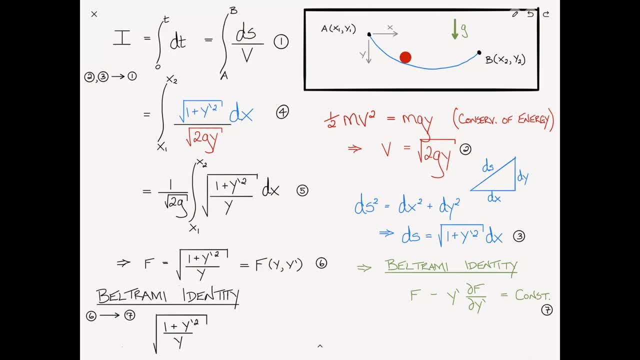 and this gives me f, which is just square root of 1 plus y prime, squared divided by y minus y prime, times partial f, partial y prime. Well, we can take the 1 over root y out, since that's constant with respect to y prime, and then we get 1, half 1 plus y prime, squared to the power of. 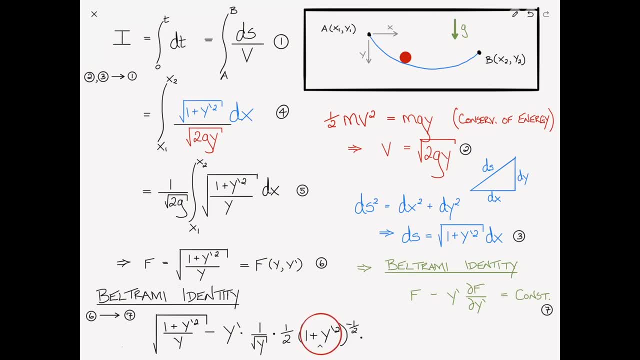 minus 1 half. Then we need to take the derivative of the inside and that gives us just 2 y prime and that's equal to a constant which we'll call c Equation 8.. Turning the page, we can simplify this equation as root. 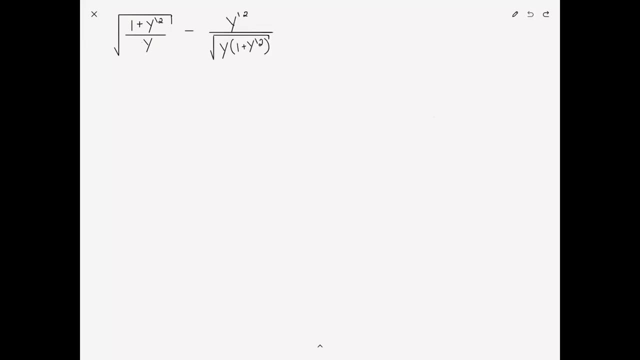 1 plus y prime squared divided by y minus y prime squared divided by root, y times 1 plus y prime squared, and that's equal to a constant Number 9.. The first thing I do is I multiply everything by the square root of y. I end up with 1 plus y prime squared, minus y prime squared divided by 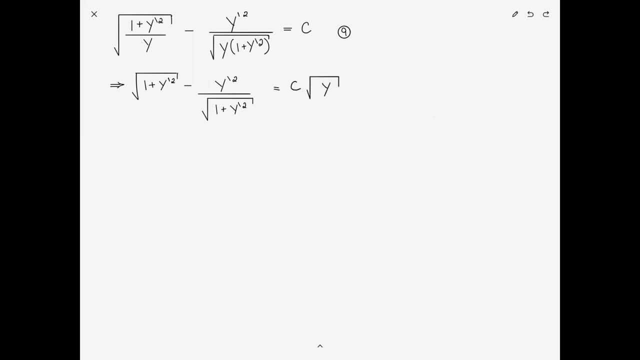 root 1 plus y prime squared and that's equal to a constant times root y. I'm now going to multiply through by 1 plus y prime squared to clear the denominator. The first term just gives me 1 plus y prime squared. The second term I just end up with. 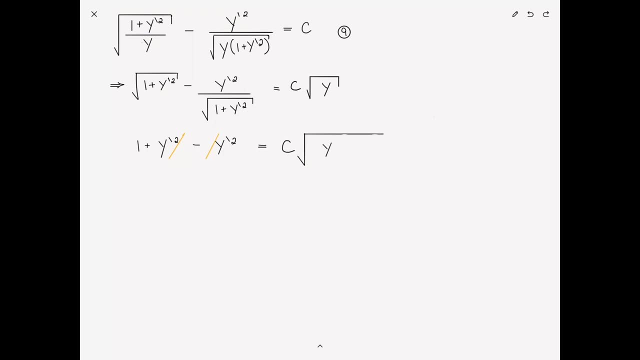 minus y prime squared, and this equals c times root, y times 1 plus y prime squared, and that is equation 10.. In order to clear the square root, we can square both sides. The left is just simply 1.. The right becomes c squared times. what's under the square root sign. so y times 1 plus y prime. 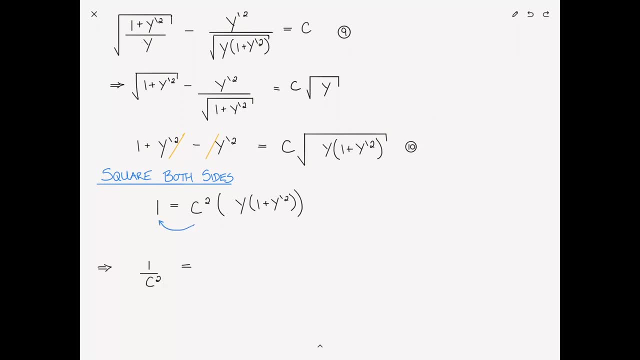 squared. Now I can divide both sides by c squared, I get 1 over c squared and I'll designate as a new constant that I'll call c1.. This is just a constant and that is equal to, if I distribute it, y plus y times y prime squared. I can rewrite this in terms of y prime. 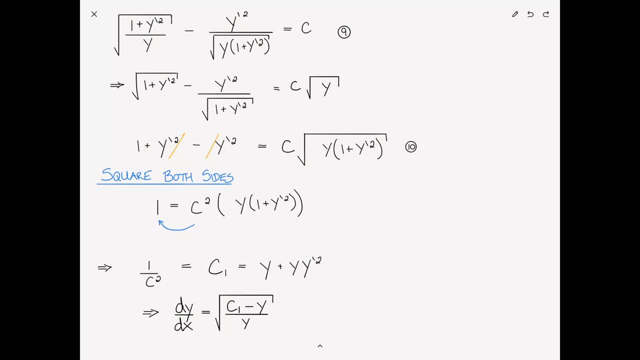 which is of course just dy dx, and that's equal to the square root of c minus y divided by y. Just simple algebra. and that is equation 11.. Next we'd like to take everything with an x to the one side and everything with a y to the other side, so that gives us: dx is equal to root y. 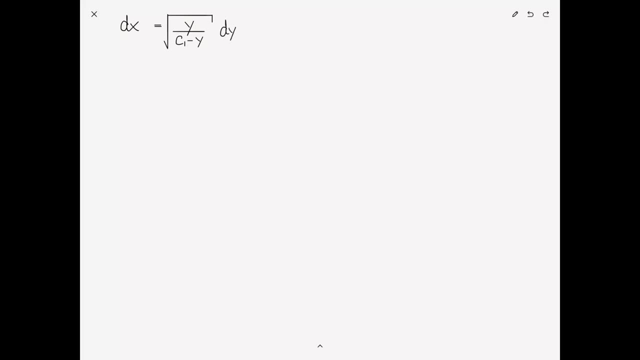 divided by c1 minus y, dy. Now what do we want to do? We want to integrate both sides. The left hand side, dead simple, just x plus a constant. We'll call this c2, since we've already used c1.. On the right hand side, let's just leave this in integral form, for now It's equal to the integral. 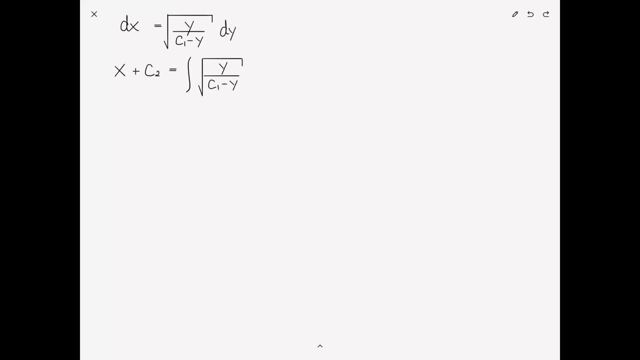 of square root of y divided by c1 minus y, dy. and now, in order to integrate this bad boy, we need to make a useful substitution. We just substitute: y is equal to c1 sine squared theta. In this case, theta is between 0 and pi by 2, and taking the differential of both sides, we get: 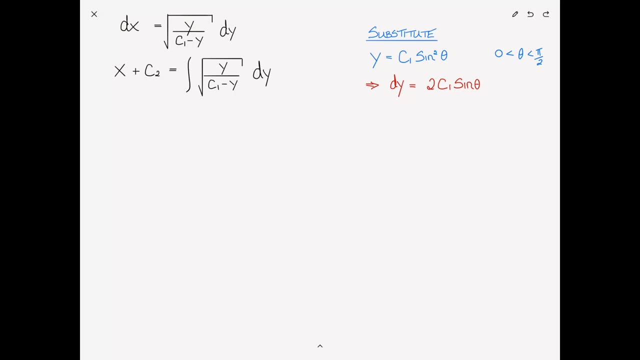 dy is equal to 2c1 sine theta times. the derivative of sine theta is cosine theta d theta. Let's give these some numbers: 12, 13, 14 and 15- and now what we'd like to do is substitute 14 and 15 into 13.. 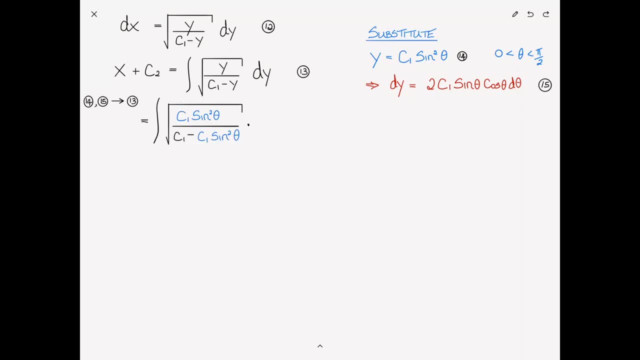 Making that substitution yields the integral of root c1 sine squared theta divided by c1 minus c1 sine squared theta, where I've just substituted for y, and that is times dy, which is all of that, Number 16.. We recognize that what's in the denominator here using a trig identity can. 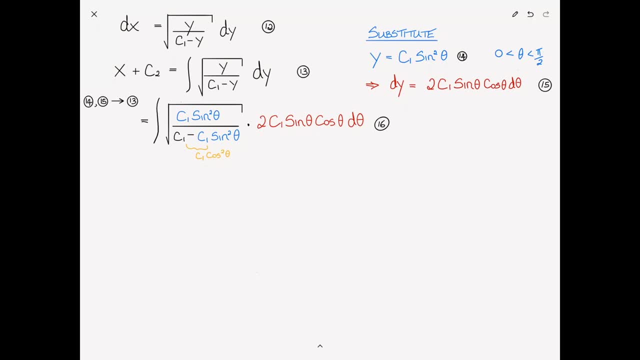 be written as c1- cosine squared theta, because we know that 1 minus sine squared theta is cosine squared theta. Now the c1s cancel, so what's left under the square root sine is just sine squared theta divided by cosine squared theta, so that reduces to sine theta divided by cosine squared. 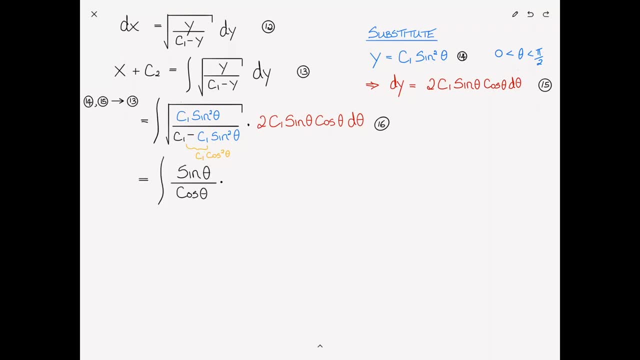 theta So that reduces to sine theta divided by cosine squared theta, So that reduces to sine squared theta times the rest of it. The cosines cancel and the sines multiply and we end up with the integral of 2c1 times sine squared theta d theta. Using another trig identity, we can rewrite: 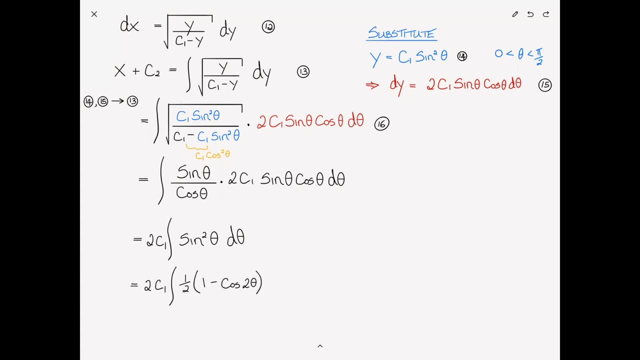 sine squared theta as one half of 1 minus cosine 2 theta. We need a d theta and now this is easy to integrate: That's equal to c1 times theta minus one half of sine 2 theta, and that's number 17.. 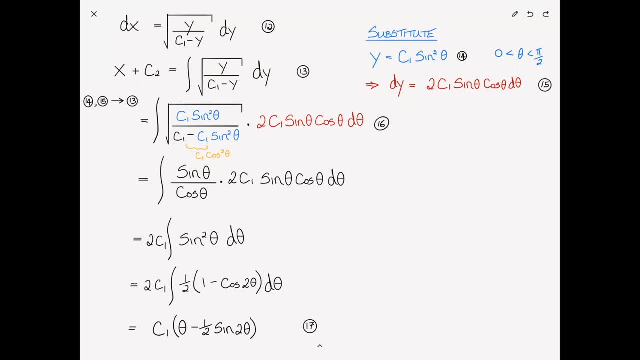 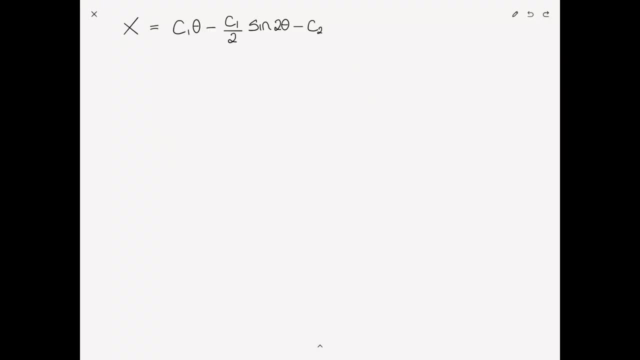 Okay, I hope I'm not losing you guys, because we're just about there. I can now rewrite equation 17 in terms of x by just taking c2 to the other side. Do that on the next page and that gives us: x is equal to c1 theta. just multiplying it out: c1 theta minus c1 over 2. 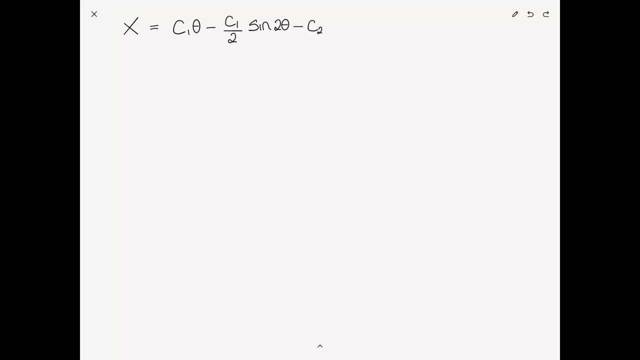 times sine 2 theta minus c2.. And we also have an equation for y. Remember this comes from equation 14 where we made the substitution: y is equal to c1 sine squared theta, which can be rewritten as c1 over 2 times 1 minus cosine 2 theta. So that's equal to c1 sine squared theta, d theta. 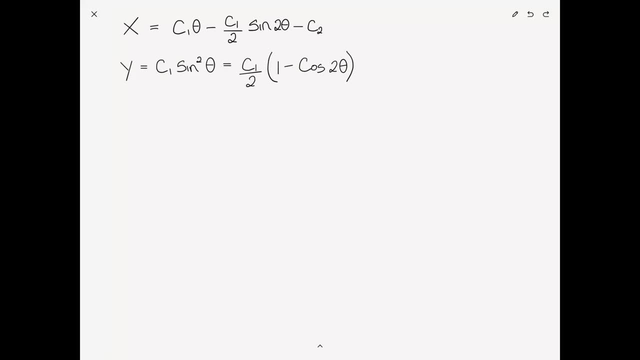 Using a trig identity, and that's it, we're done. Let's put a red box around that, give it some numbers, and then, of course, c1 and c2 can be found using the boundary conditions. Now, these equations, 18 and 19, are known to be equations for a cycloid. It's a shape known as a cycloid and this is the 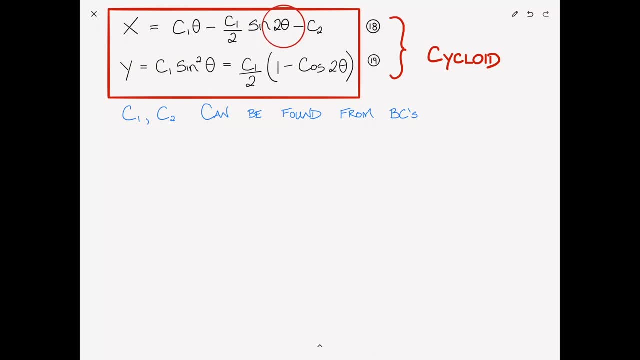 parametized form of the cycloid equations, because it's written in terms of the parameter theta. What is a cycloid? Well, if we take a straight line and we roll a disc or a wheel along that, if we mark a point on the perimeter of the wheel as that wheel rolls, a cycloid is the path traced. 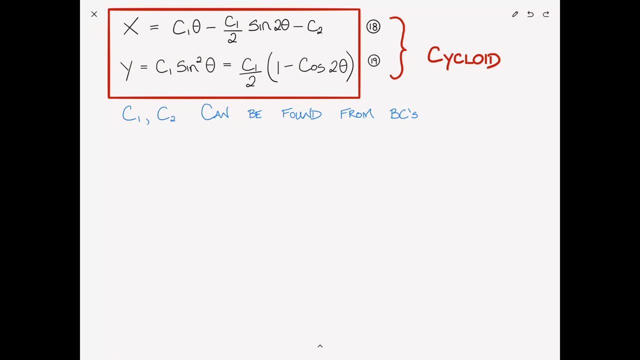 out by that point Looks something like that, And then I was able to find some graphics online that further illustrate this. So a cycloid is the shape that this point makes while rolling along a straight line. If it was rolling along a curve, it would be called an epicycloid or a hypercycloid, depending. 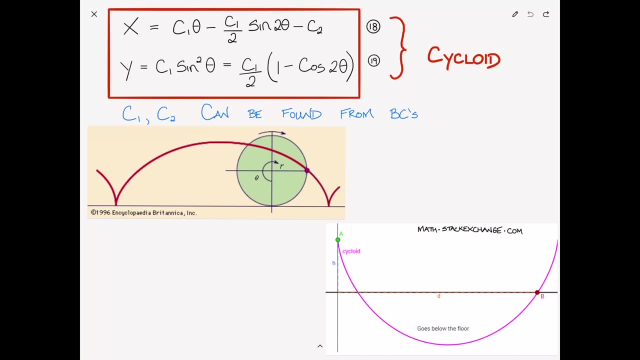 on whether it was inside or outside the curve. And going back to the original problem, which was trying to find the fastest path From point A to point B, The answer is it's the cycloid through those two points. So this cycloid curve from point A to point B represents the minimum time curve. And what? 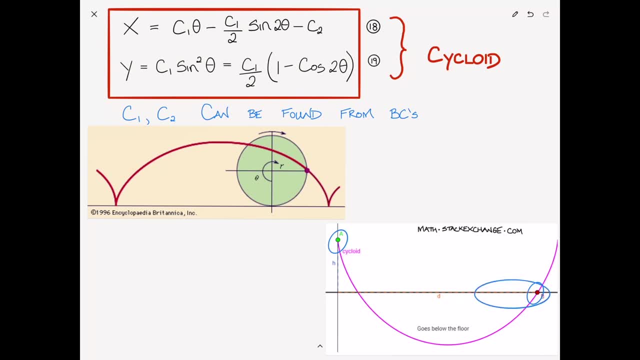 might be interesting to some of you is if this were ground level. here, where point B is the minimum time curve, is actually a curve that goes underground and back up again. All right, so we're done with this. This is the brachistochrone problem and this is what prompted 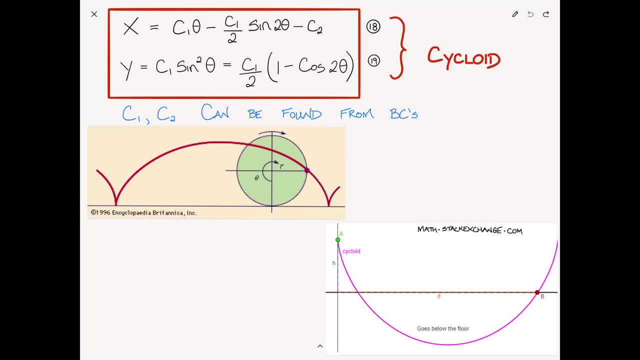 the discovery of the calculus of variations. It took about 60 years, from the time-burned calculus of variations to the time Euler published the calculus of variations. One can only imagine how much quicker all of this would have gone if these guys could have jumped on a zoom session. 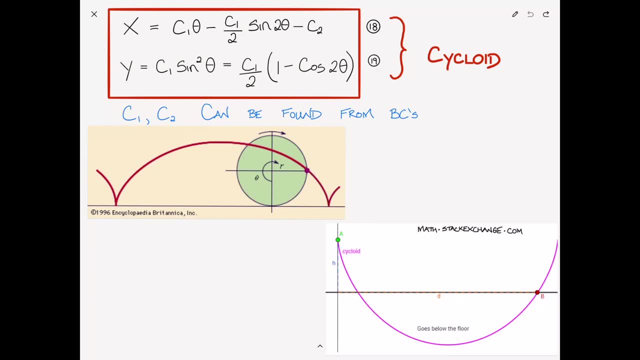 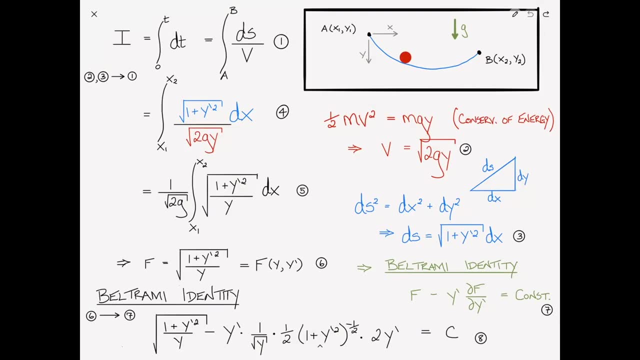 and done a screen share with one another. Before we go, I want to take it from the top one more time and just review this really quickly. We solved this problem by using the calculus of variations, which requires us to find an integral that we're trying to minimize. In this case, the integral was a minimum time integral, which we could 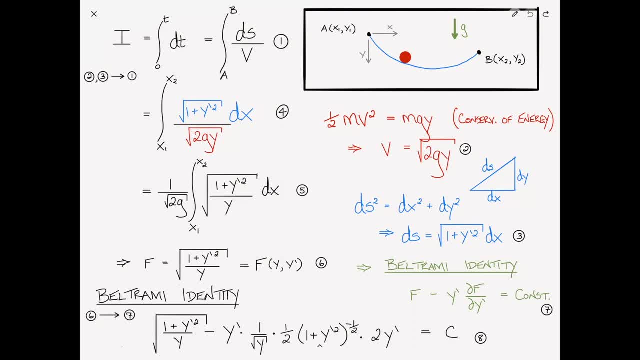 write in this form: ds divided by the velocity, and that gave us this final form. From that form we identified the functional. We recognized that because the functional doesn't explicitly depend on x, therefore we can use the Beltrami identity. That's the form that the Euler-Lagrange equation 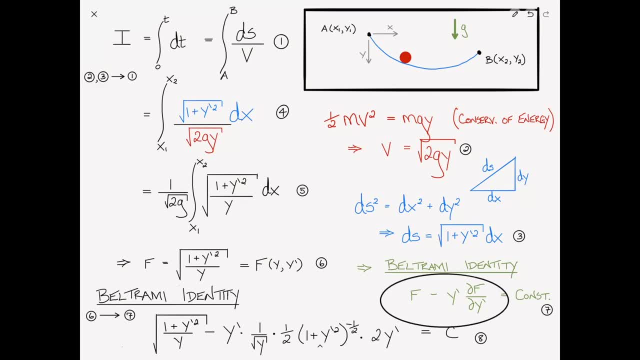 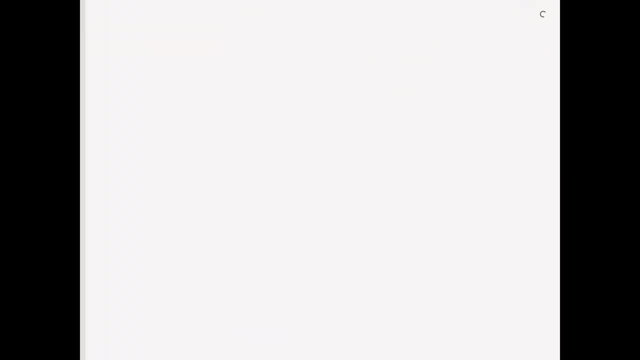 reduces to. in this case, We substituted our functional into the Beltrami identity, We integrated it by making a substitution over here And when we performed the integration, we ended up with an agreesal equation describing a cycloid. Before we leave, I mentioned, I would talk a little bit about the